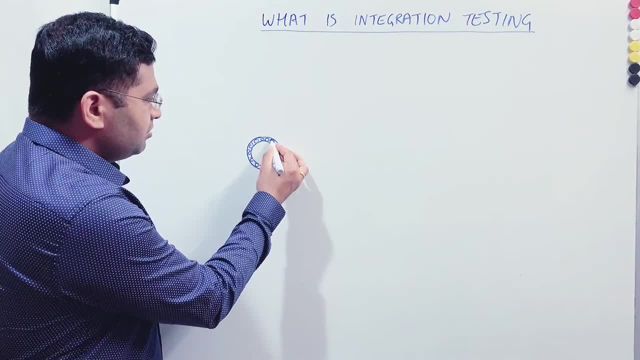 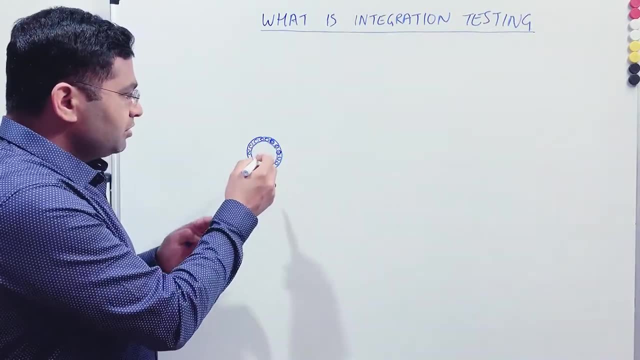 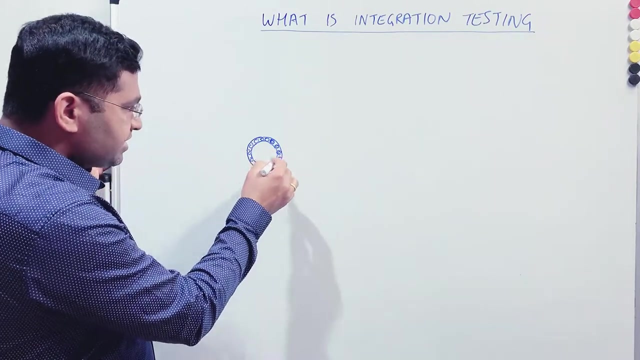 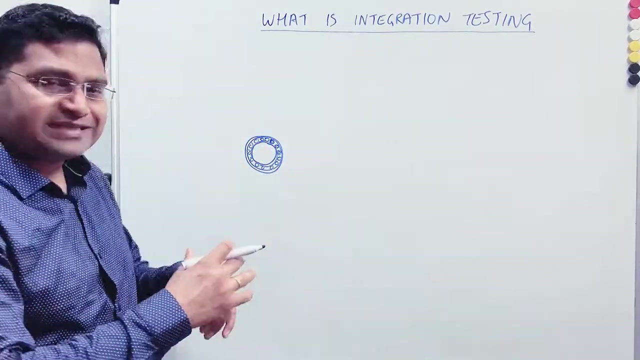 etc. right, So these are, you know, metal balls, basically you can say, of very small size that fit into the ball bearing, all right, And once you tested these, and then these are assembled within the, within the metal frames that are there. so these two frames, then that becomes assembled unit, or 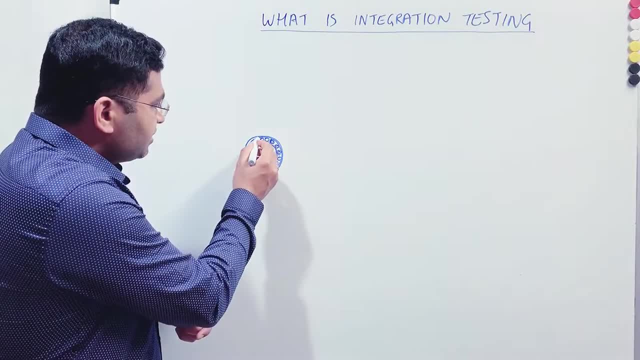 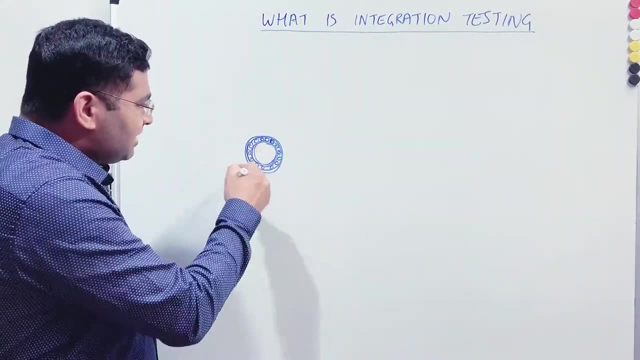 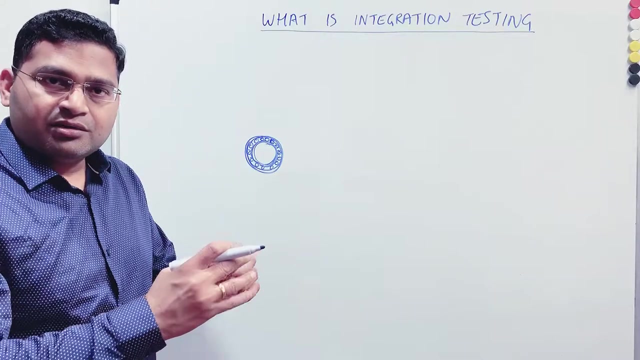 integrated unit. right, Because these units are integrated with the upper and inside layer right. So those are two other separate units. So this had made a ball bearing together. Now this is an integrated unit which can be tested, you know, separately or as an integrated system. 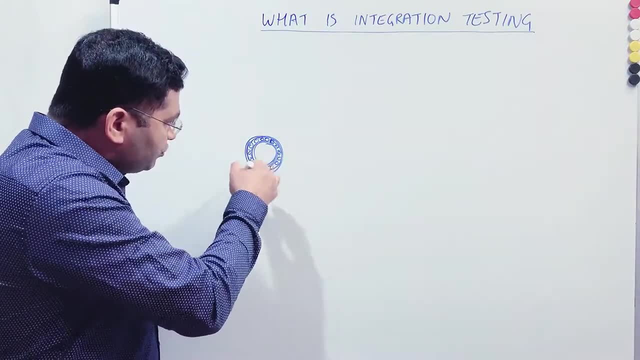 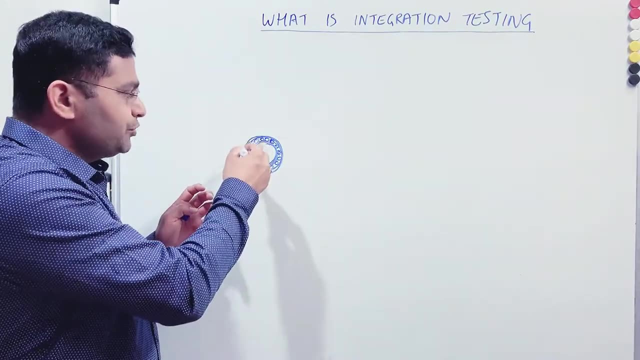 or integrated ball bearing, All right. So now, when you are testing this ball bearing, that becomes integration testing. okay, You have integrated different units that made that ball bearing or that make that ball bearing and you are testing it, right. 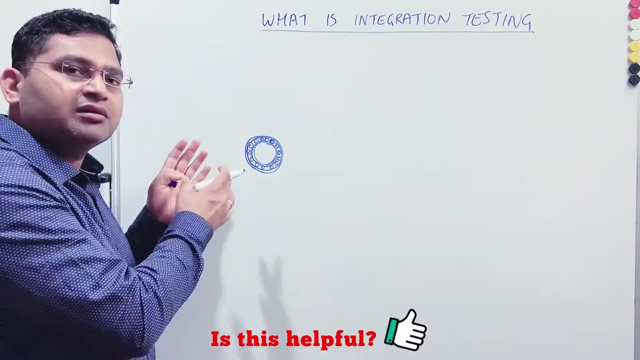 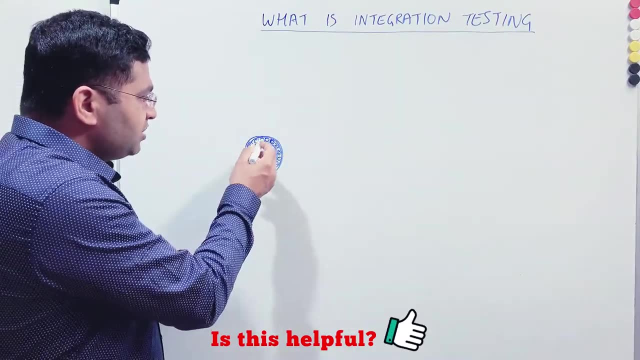 So this is what integration testing is in the car space or in the actual, you know, car manufacturing. So when you are testing it Now, this ball bearing, there will be, you know, rim on top of it when you integrate the rim. 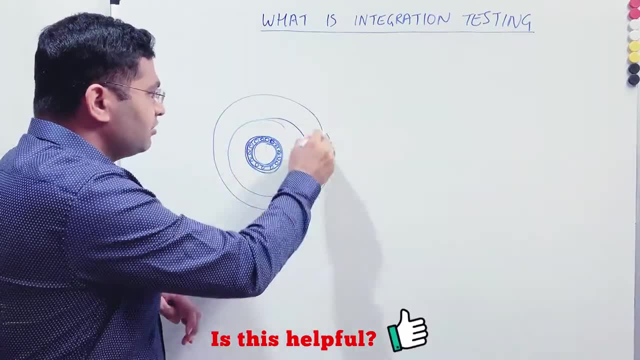 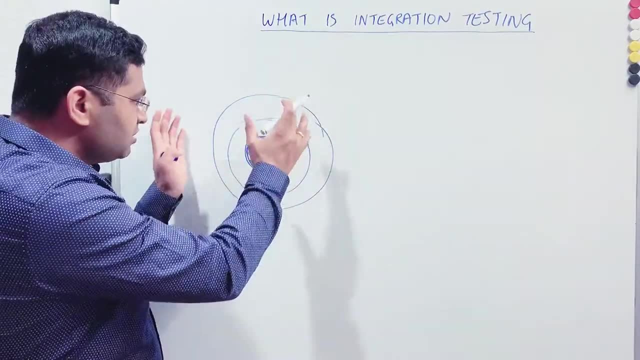 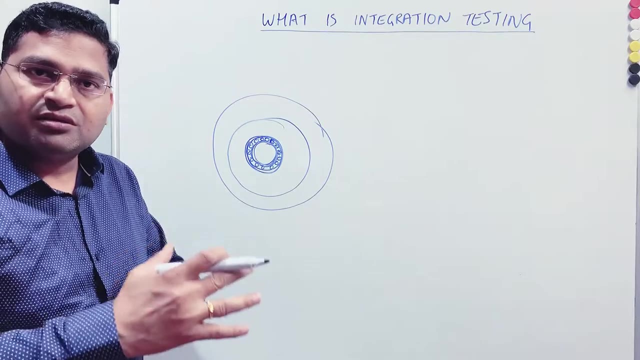 Then you test that whole part, Then you will have the tire on top of it, right. So now, this is what the overall wheel becomes of a car. Now, this is, you know, an integrated system, or a wheel that gets tested at each and every integration phase. 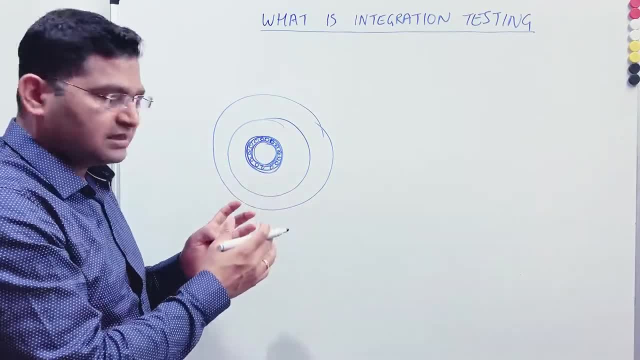 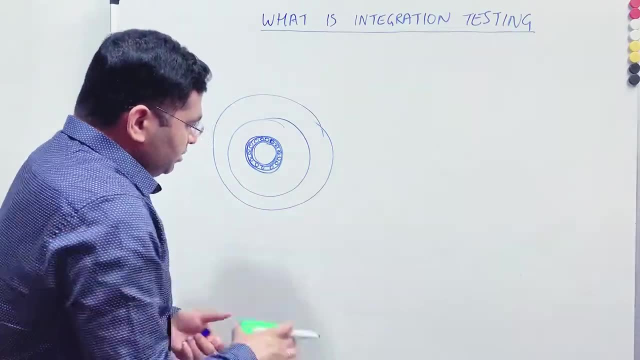 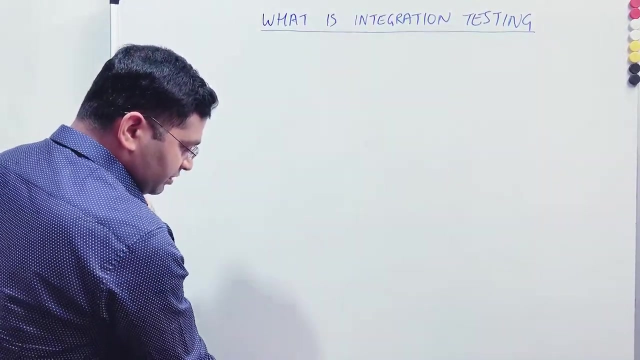 Right, so once this bearing is integrated with the units, it gets tested. then it gets tested along with the rim, and then along with the tire, etc. right So, this is what the integration testing will look like into the car manufacturing space, right so? 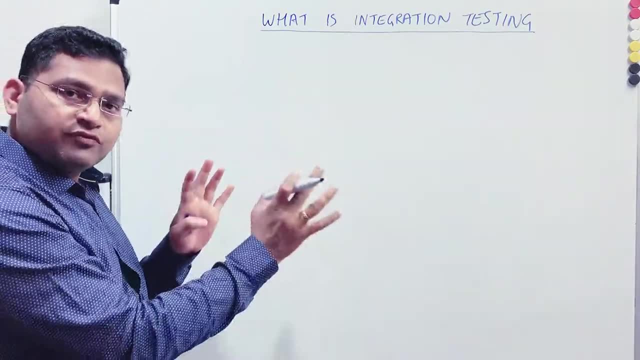 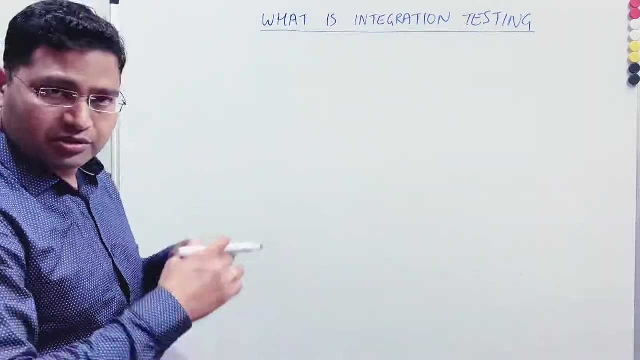 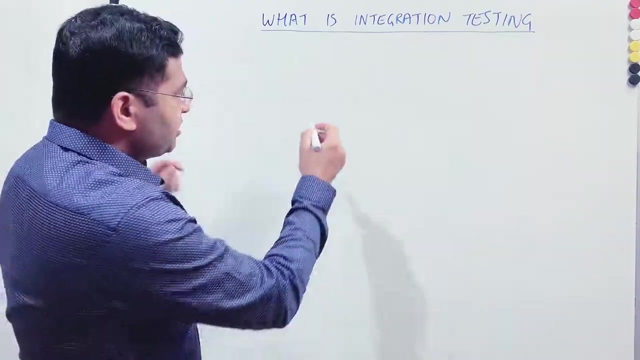 this is testing one tire. once the tire are applied, all the four tires are applied. so this is how the approach will happen in the integration testing of the tire or the car, now correlating that with the software. okay, so we have understood of the e-commerce website. so e-commerce website will. 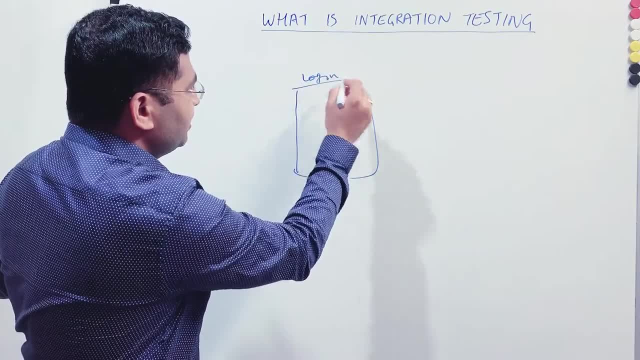 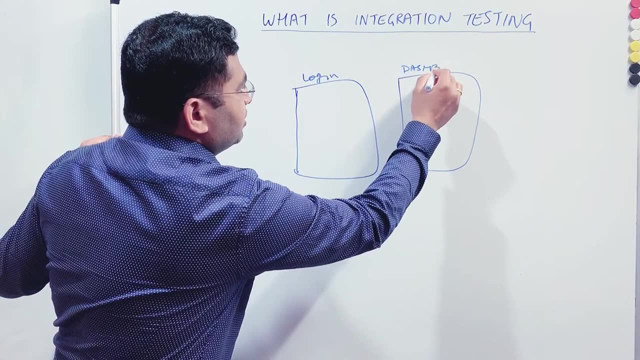 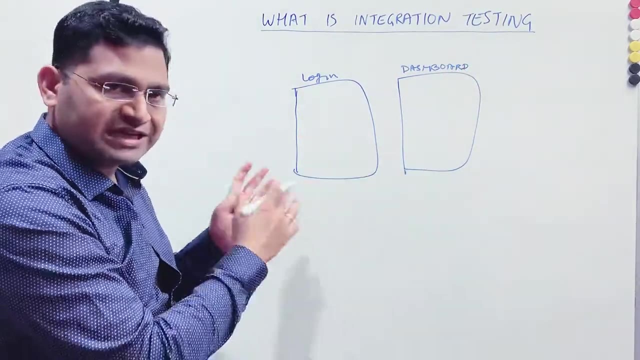 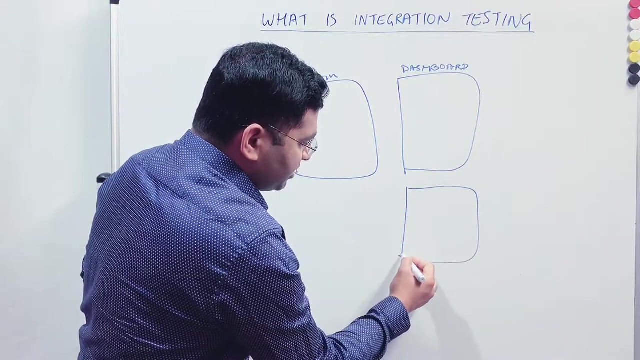 have separate modules, so we'll have the login module right and then, once they use a logs in, then he might be redirected to the dashboard, okay, where he will find all the information about his previous order. you know his profile information, address and everything. then he'll have you know by items. you know buy items capability. he can go to checkout, all right. 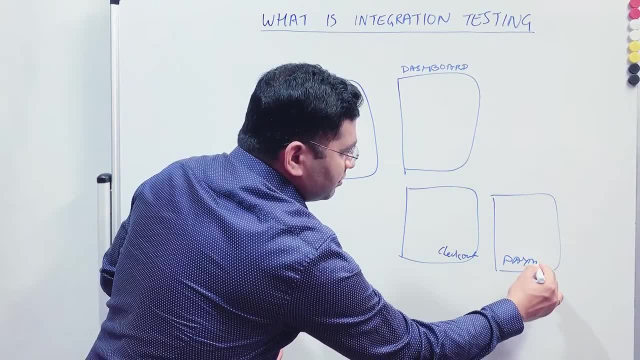 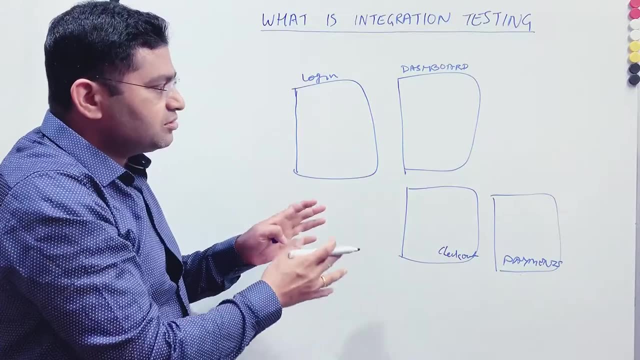 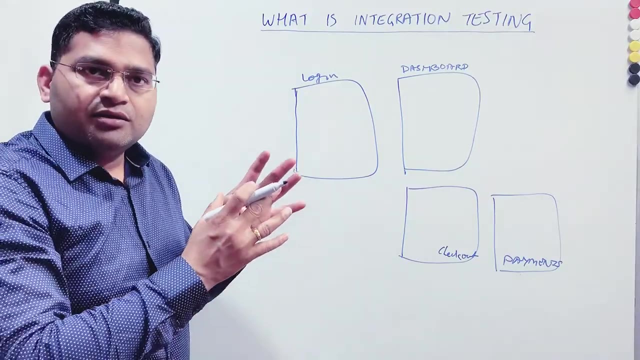 he can go to checkout. all right, then go to the boy direito automation. okay, then you start running, can do the payments, so payments page, okay. so these are some of the you know functionalities or high level functionalities that can be there. now these are integrated. you know these all. 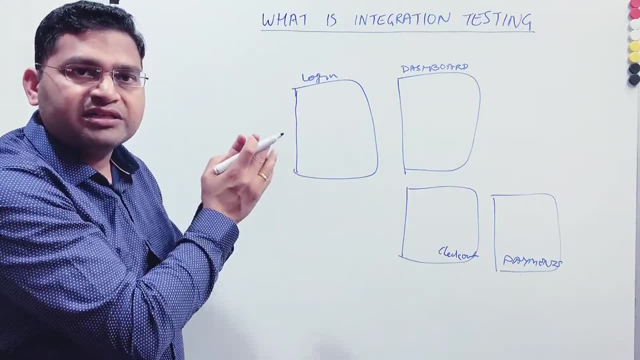 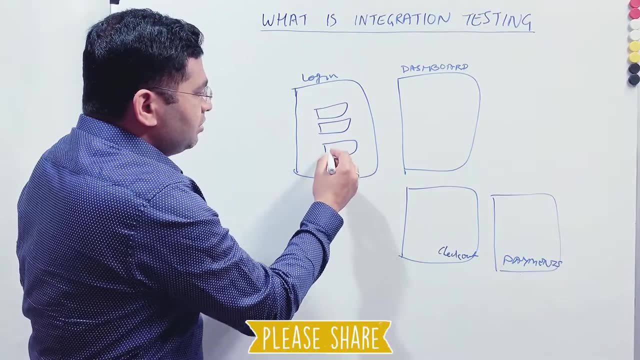 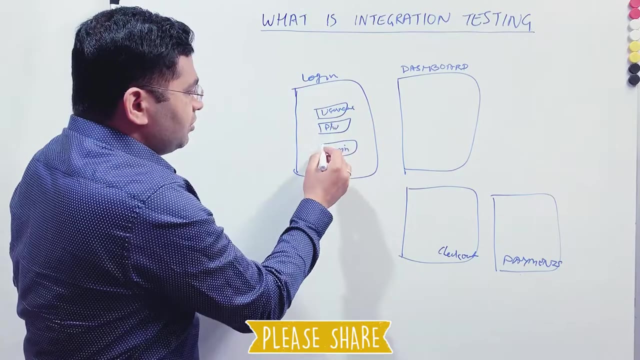 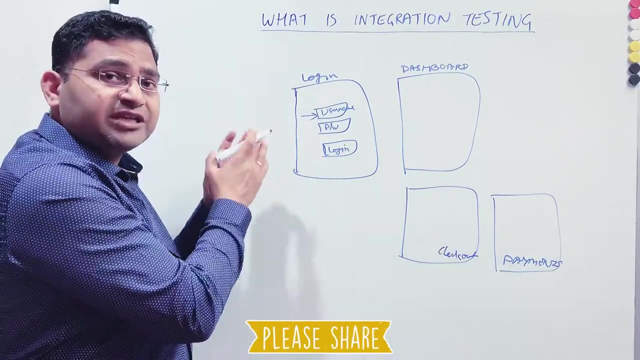 different modules that you see or the functionalities that you see are integration of the smaller units. now say, for example, login page will be having username, password and the login button. all right, so password, username and a login button. okay. so username is one of the unit, could be one of the unit if it is 10, if it can be tested independently, right then you have the password. so 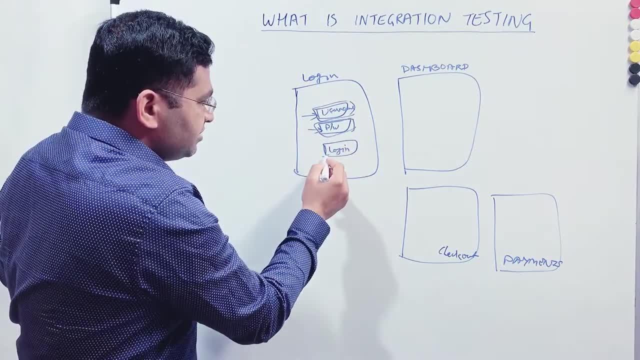 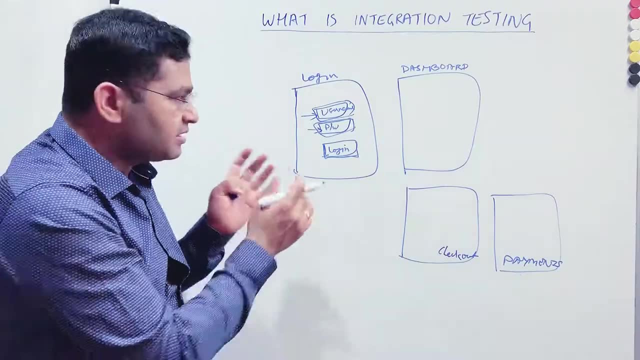 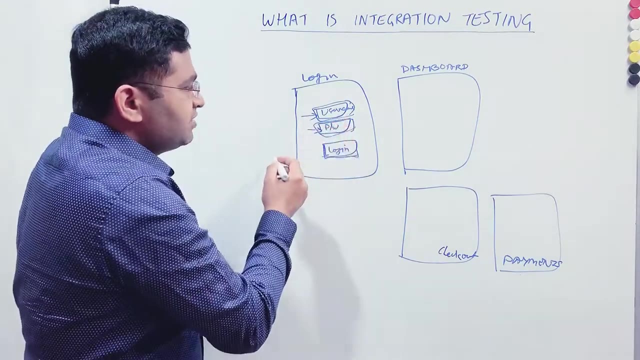 username and password and then there is a login button. that has been implemented on this page and there has been some integration of business logic being built when this username, password login button has been added on the login page. for example, when user enters the username and password and clicks on login button, then after successful login, user will be redirected to the 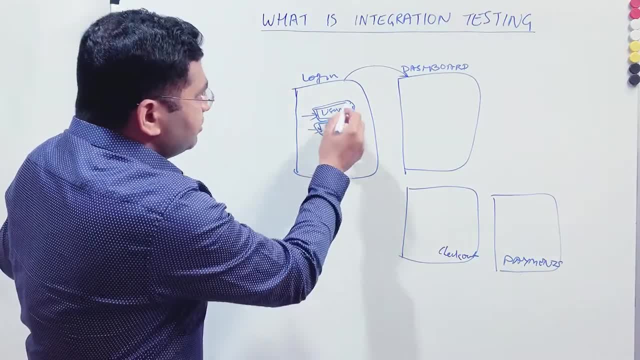 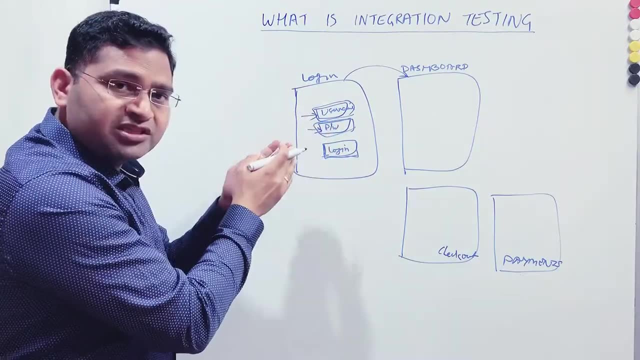 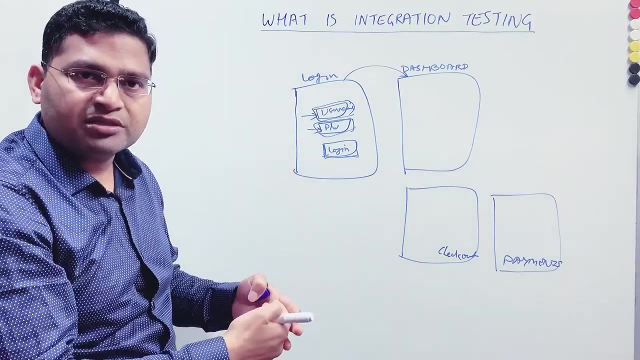 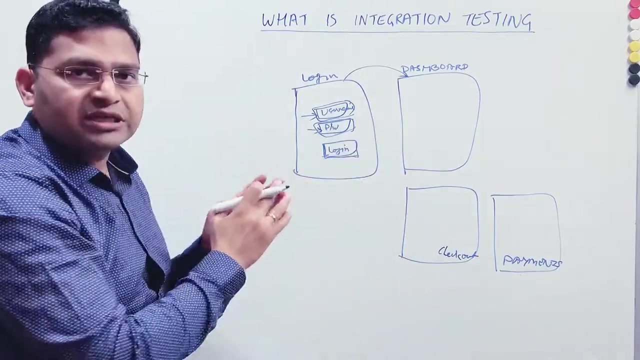 dashboard right. so when the testing happens with the integration is placed. for example, in this case, if you are testing the login page, which has username and password, and you provide the password and then after logging, but logging in, user is redirected to the dashboard. this is what integration testing is, because you are not testing the individual units as such, you are testing the.